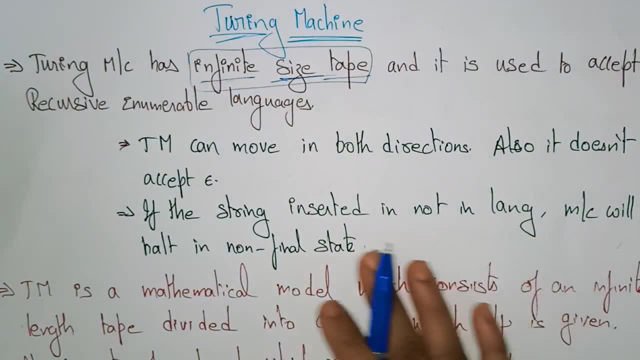 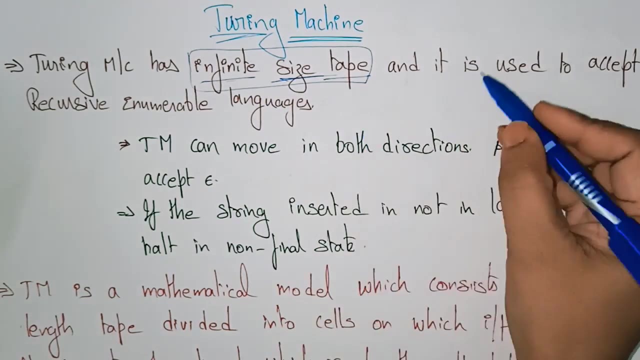 automata. this is also an infinite size tape we are using here and it is used to accept the recursive. Recursive means the same set of rules, or repeating- Okay, and enumerable languages means some set of items, set of elements, Okay. so the Turing machine has an infinite size tape, A tape. 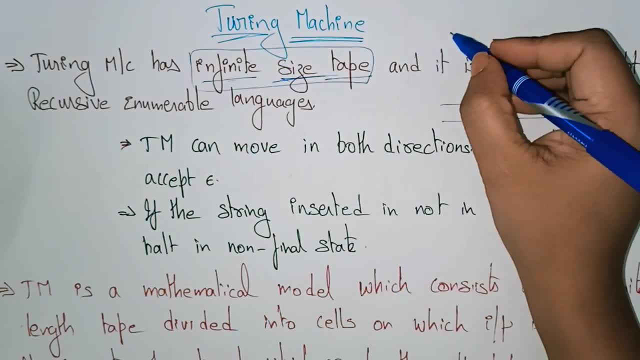 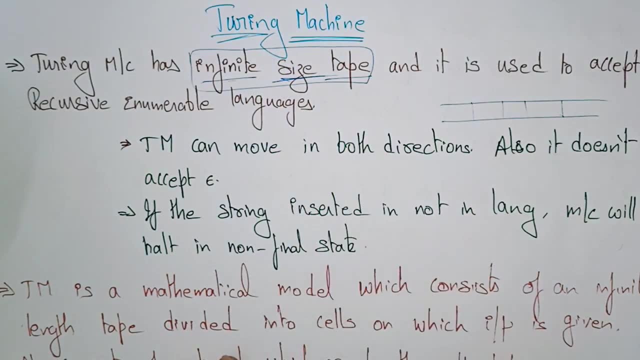 here we are using a concept tape. So far in the pushdown automata, whatever we have seen, that is a stack concept we are using. But here in the Turing machine, you have to remember that we are using the concept tape instead of stack and it is used to accept the recursive enumerable languages. 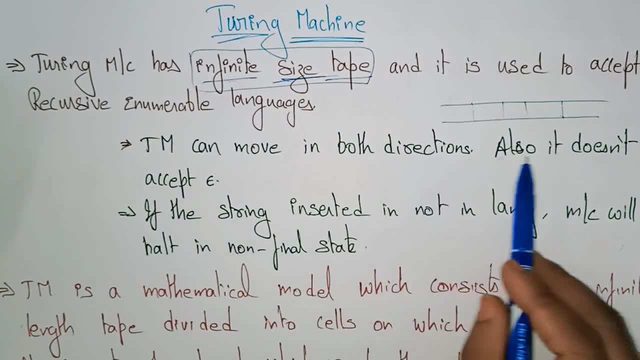 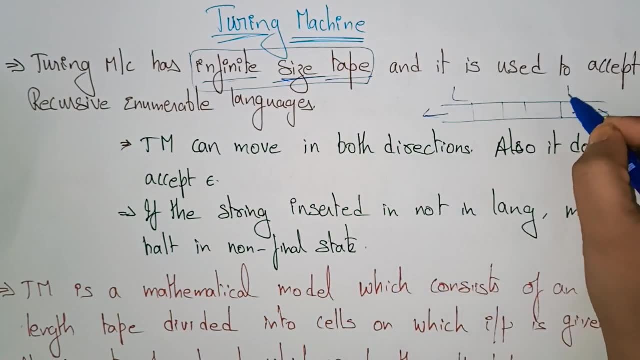 A Turing machine can move in both the directions. Also, it does not accept anything, So it is used to accept the recursive enumerable languages. Okay, it can move in both the directions, either to the left side, either- it has to- to the right. 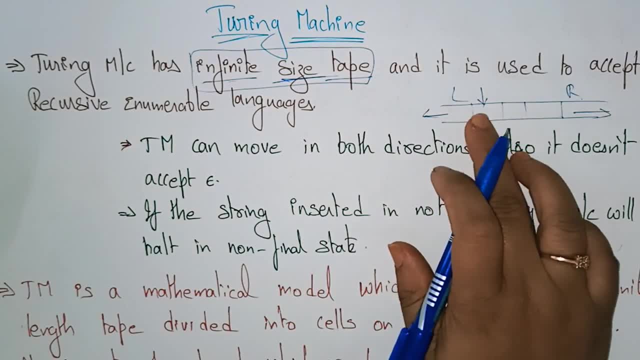 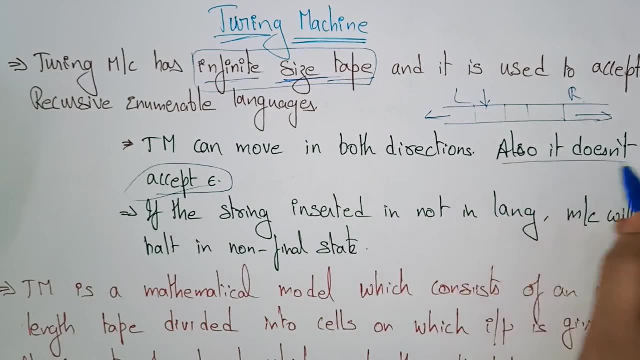 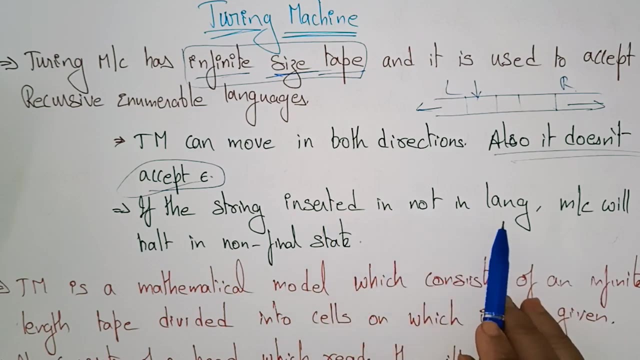 side A tape consisting of some head. Okay, that head can move towards right, or can it move to towards left, but it does not accept the epsilon. does not accept the epsilon. If the string inserted in not in, the language machine will halt in non-final state, Suppose, whatever the string. 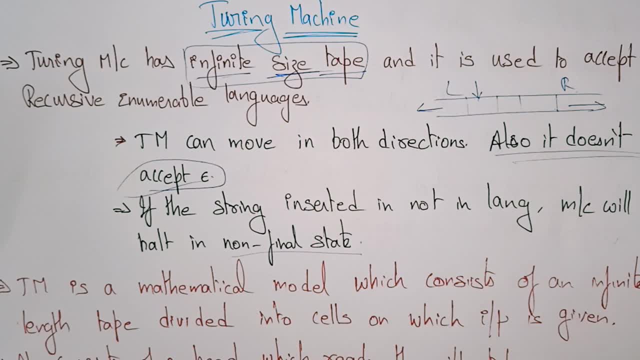 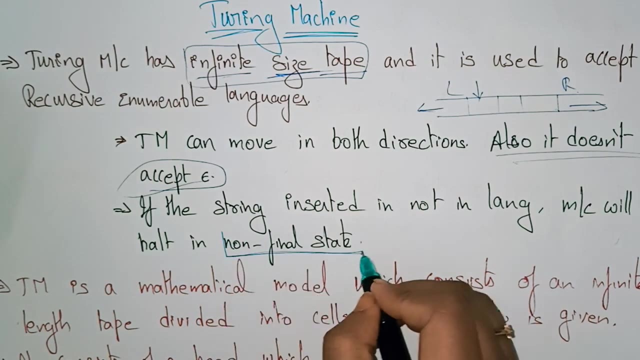 that we are want to be conduct means a Turing machine. it has to check whether the string is accepted or not. If the string inserted is not in the language, if it is not present in the language, then the machine is becomes halt in non-final state. Okay, suppose if the string is accepted it is in the language. 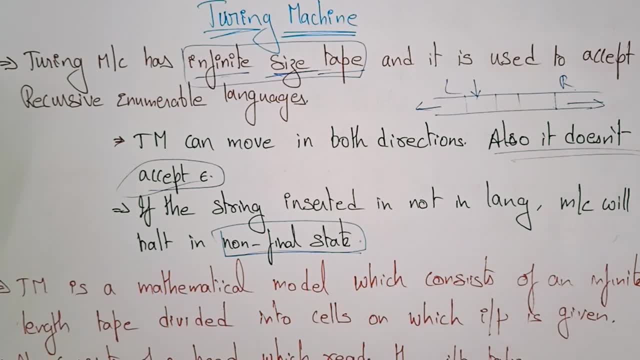 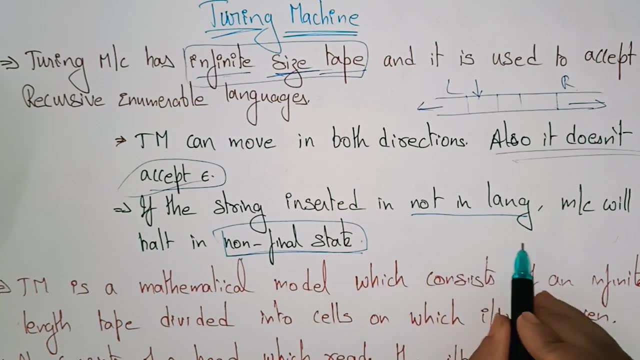 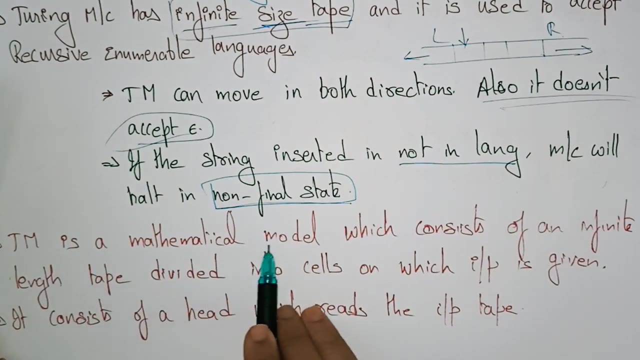 if it is present in the language, the machine will also halt, but in final state. If not in the language, means it is halt in the non-final state. If it is in the language, means it is halt in the final state, It is not in final state. So the Turing machine is a mathematical model which consists of infinite. 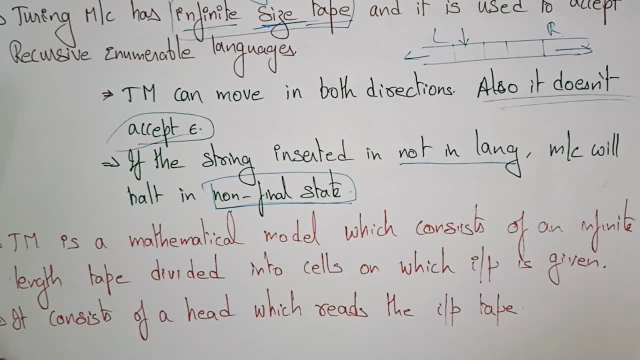 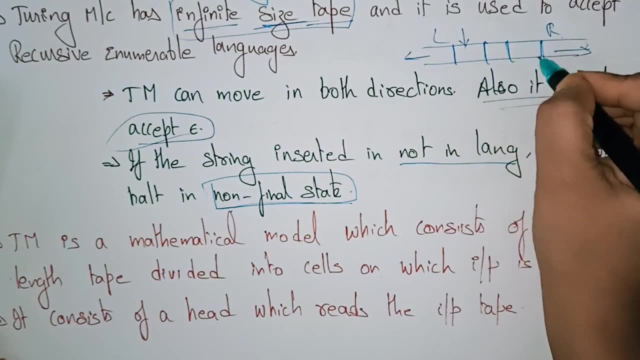 length tape. So this is the length. tape is not a constant here. It is an infinite length tape and it is divided into cells. So these are the cells. The tape is divided into cells. So this is one cell, one cell like that. So tape is divided into cells. 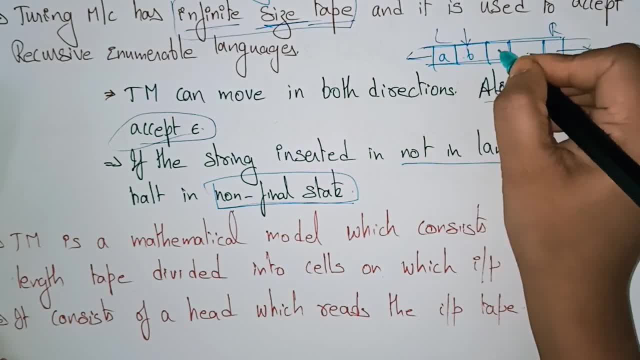 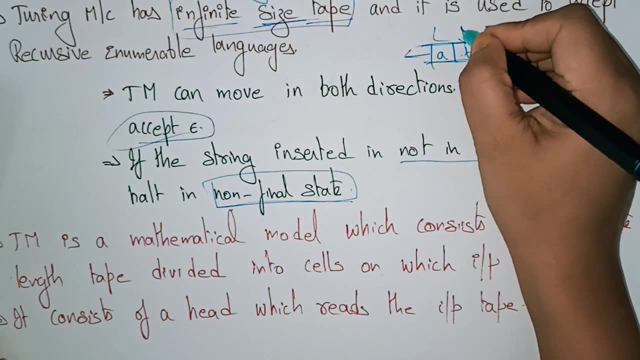 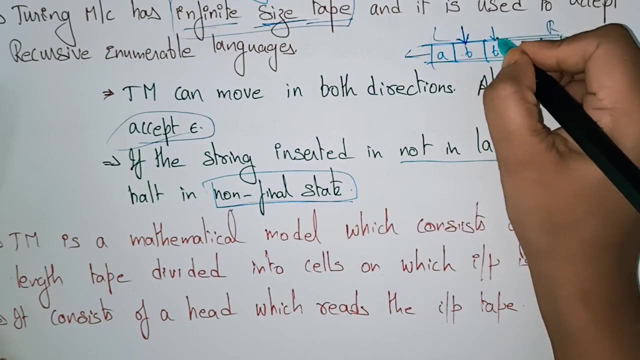 On which input is given. So here we are giving the input A, B, B, like that any string input is given. It consists of a head which reads the input tape. So this is a head which reads the input. Now. first it reading B here. So after that the head is moving, suppose right. Next it reads again: 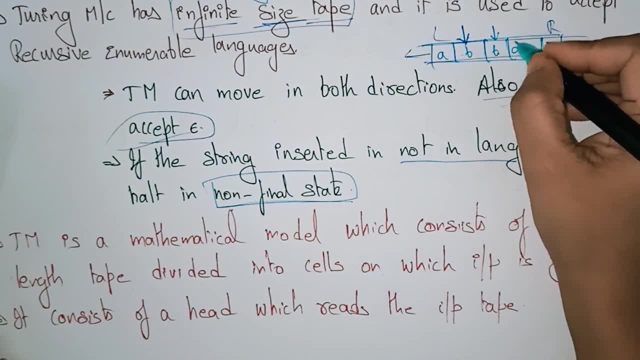 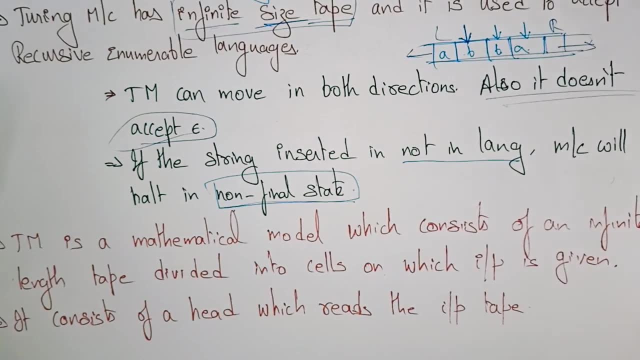 B, Again the head is moved to the right. So after reading one cell, it head moves to the right or the left and reads whatever the element that is present in the tape. Okay, so it consists of a head which reads the input. So this is the head which reads the input. So after that the head is 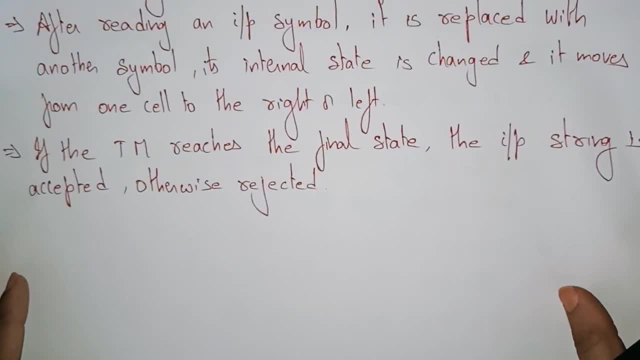 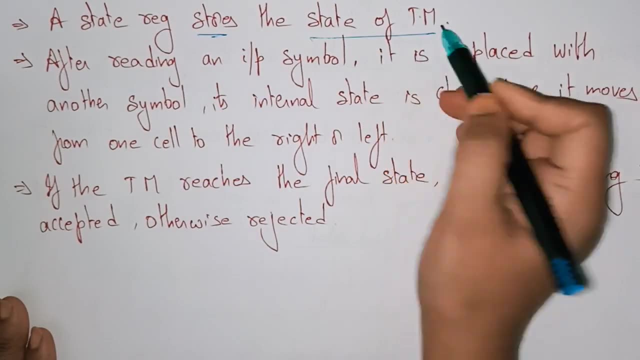 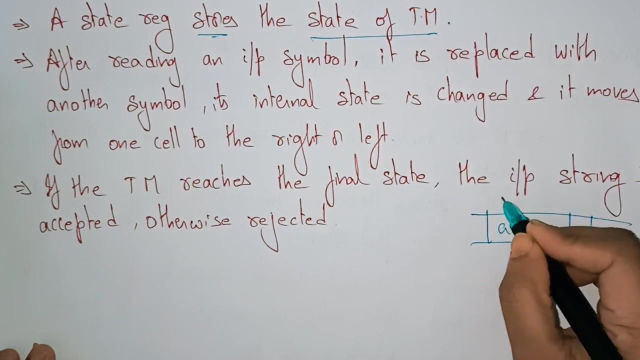 changed. So this is a head which reads the input. A state register stores the state of Turing machine. A state register stores the state of the Turing machine After reading an input symbol. so whatever the input symbol that is present on the tape. So after reading an input. 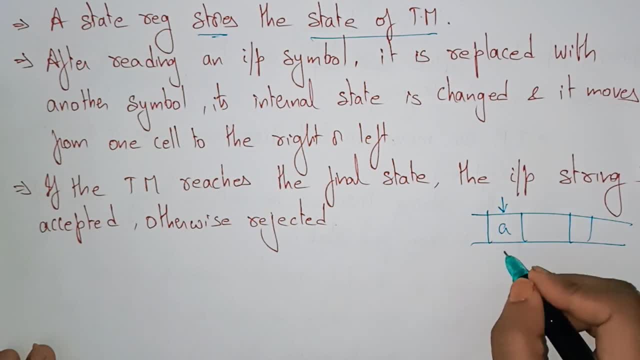 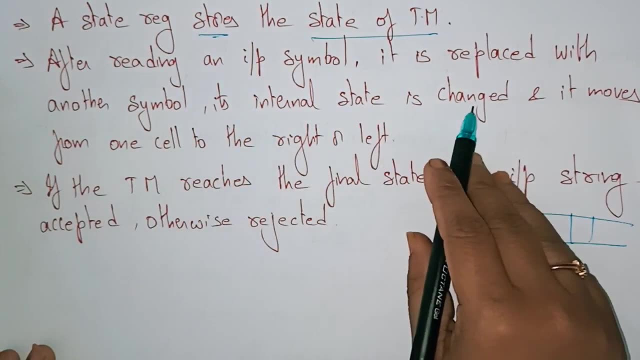 symbol. it is replaced with another symbol. Okay, replaced with the another symbol means the terminal or non-terminals. It is replaced with another symbol. Its internal state is changed. it and it moves from one cell to to the right or left internal state is also: 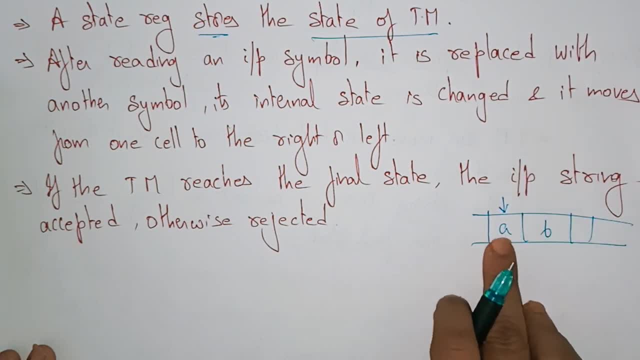 change. suppose it, if it is a and this is a B, this input symbol is replaced with another symbol, okay, and the state is: suppose it is Q, naught. suppose we are moving to the end of the next cell, in that you are getting another, a new element, new input symbol. suppose it is a, B, so the here it will be replaced with. 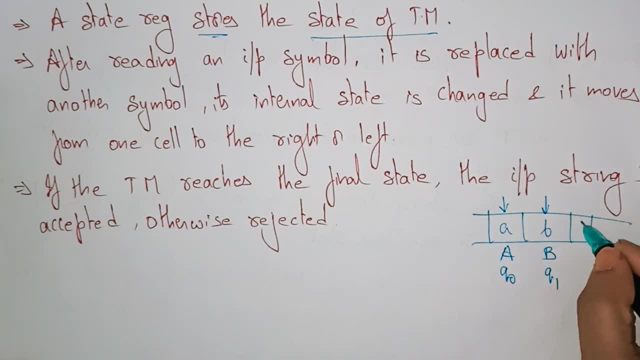 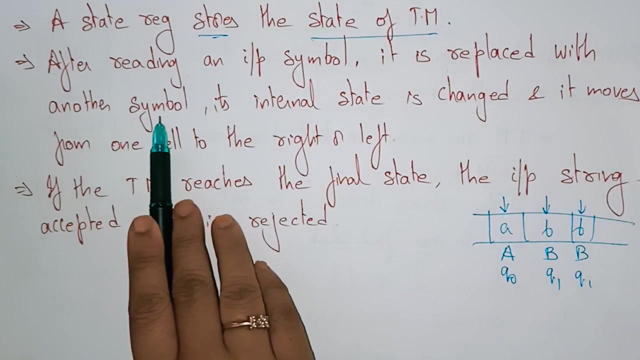 another symbol and the state will be changed to Q 1. suppose here also B is there. then the state remains the same. okay, the state will not change for the same element and it is replaced with B only like that. so after reading an input symbol, it is replaced with the another symbol and its internal state is changed. 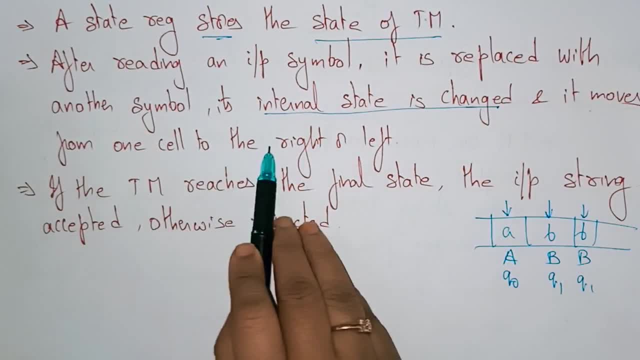 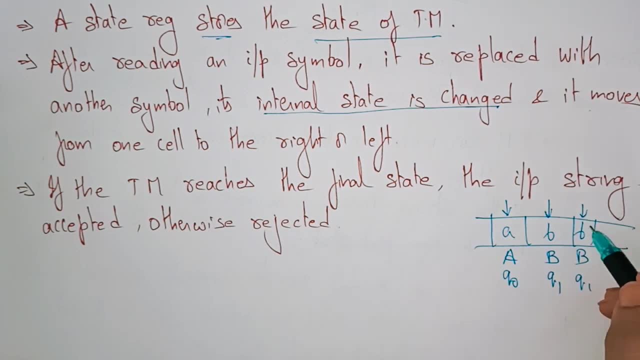 only the internal state is changed and it moves from one cell to the right, or it can move to the left side if the Turing machine reaches the final state. suppose, if it reaches, this is the final state, a B, B- that my string is only a B B. 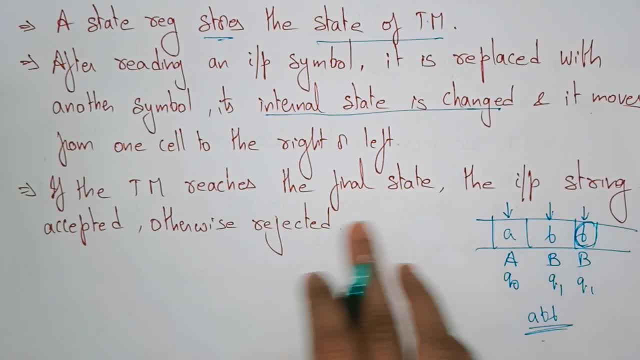 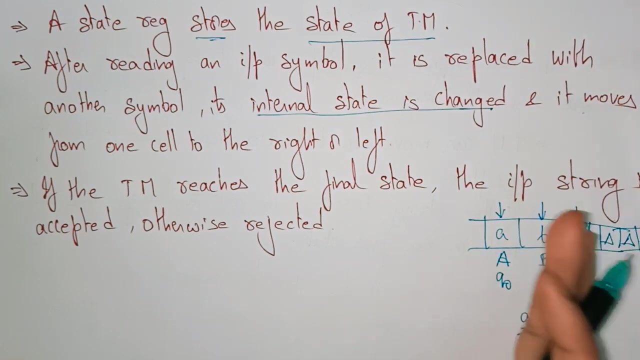 if the Turing machine reaches the final state, the input string is accepted, otherwise it is rejected. so after that it will have all the all the blank spaces, okay. so whenever we are seeing that blank space okay, we have to say that the string is accepted. if it is at, the blank space is not there, and even 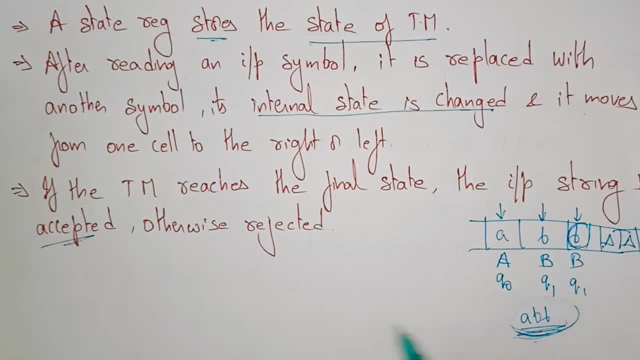 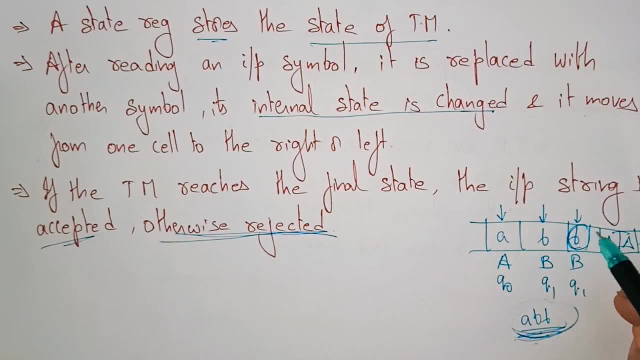 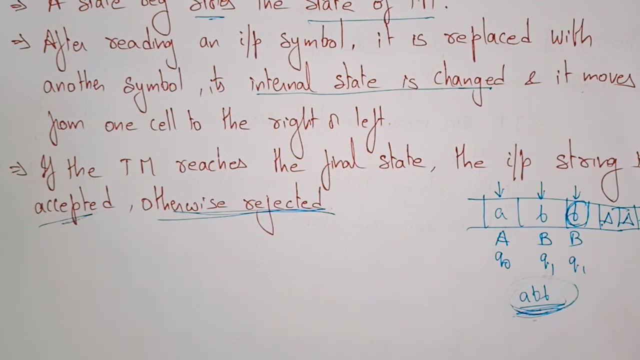 though, if you, if the string is not reached, if you didn't reach the string, then the string, the Turing machine we just rejected. whenever the Turing mission reaches the final state, the input string is accepted, otherwise it is rejected. so this is a just a concept, the introduction part of the Turing machine. 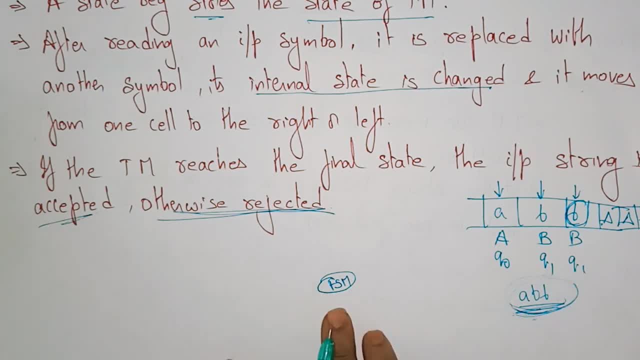 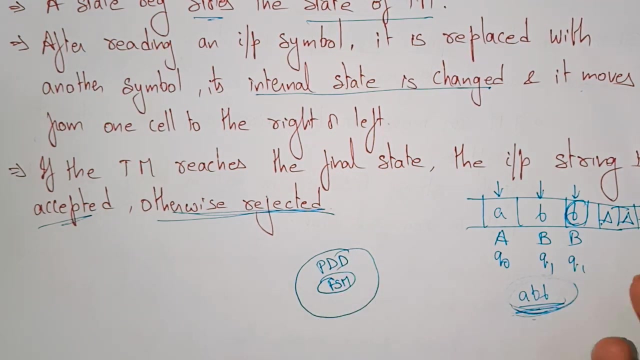 so actually the yeah, we are having the finite state machine. so far we have learned about the finite state machine. the first topic in the subject there is a finite state machine. so after that, the finite state machine- we are discuss about the pushdown order meta in the finite state machine: non deterministic. deterministic finite. 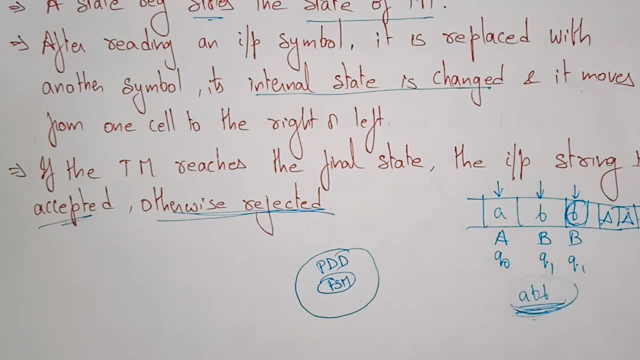 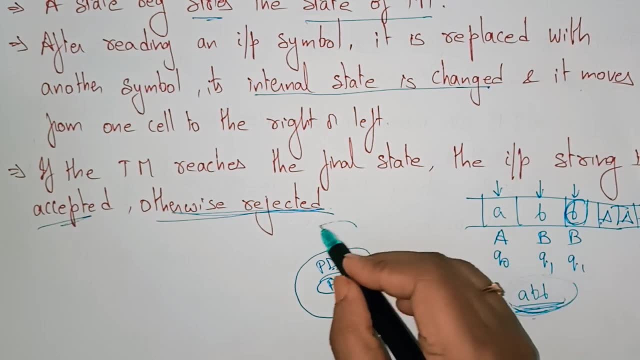 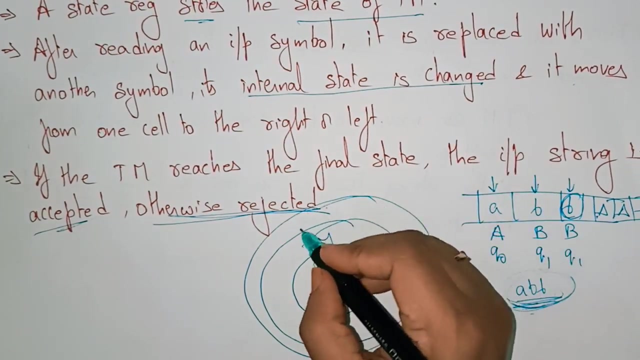 automata with epsilon, with epsilon without epsilon, melee and more emissions. we learn, and then pushdown automata. so in the pushdown automata we are discussing with some all that methods and next is a Turing machine. now we are learning about this Turing machine. after that some undecidable automata will be. 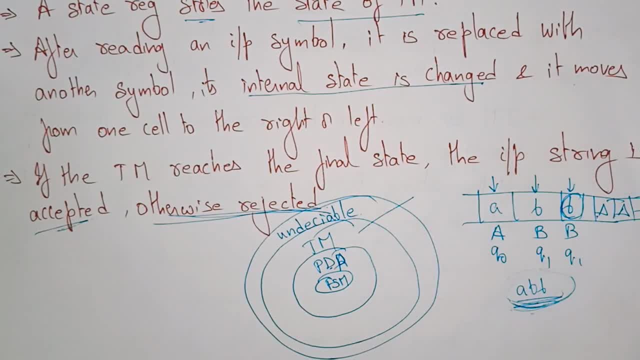 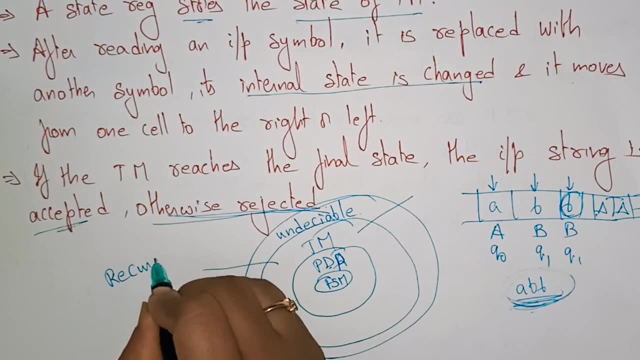 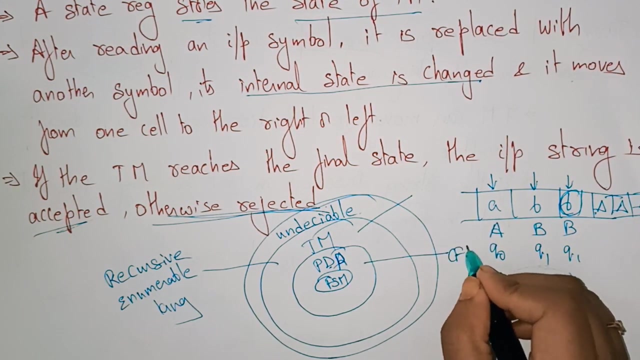 there. okay, so for Turing machine we are using recursive enumerable language, what I said now. so what I said, Turing machine is a recursive enumerable language. the language that we are using in the Turing mission is a recursive enumerable language, whereas in the pushdown automata, what language we are using? we are use the context free language pushdown. 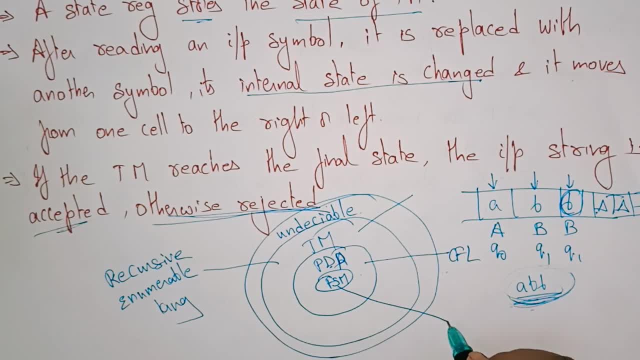 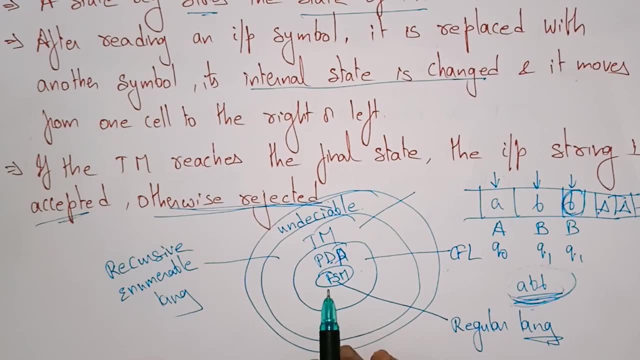 automata, we use the context free language, whereas in finite state machine we use the regular language. we use a regular language. and in finite state machine we use the context free language, whereas in finite state machine we use the regular language. we use a regular language. so remember this point in the 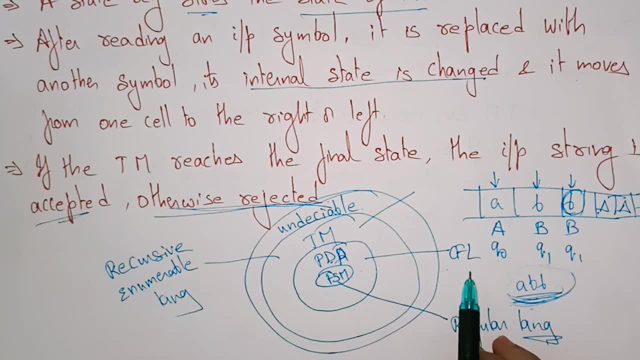 finite state machine we use a regular language, pushdown automata we use a context free language and in the Turing machine we are using the recursive enumerable language. okay, so in the next video I will explain the formal definition of the Turing machine. thank you.